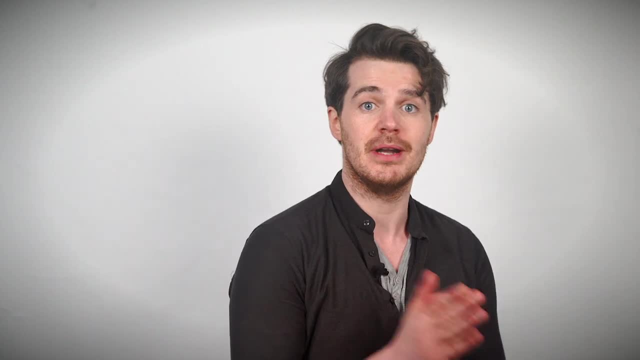 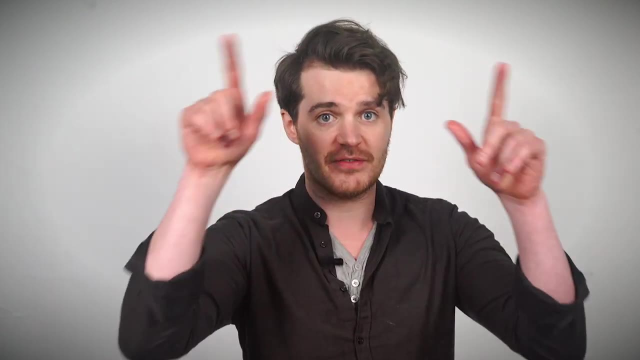 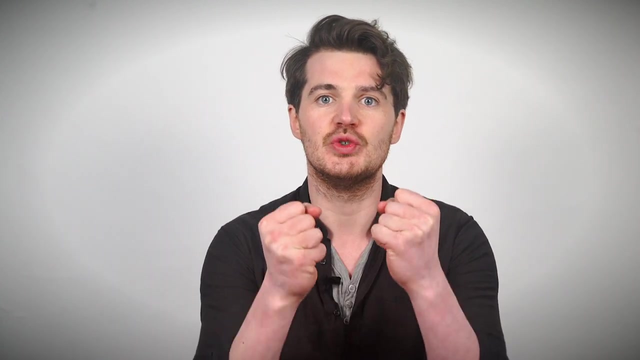 focus on the extra 150 calories that you're going to burn, saying this, while I drop the calories From the moment you wake up. you can start doing this positive framing. What I do is, instead of thinking about how much I don't like getting up in the morning, I focus on how much I do like my morning coffee Instead of 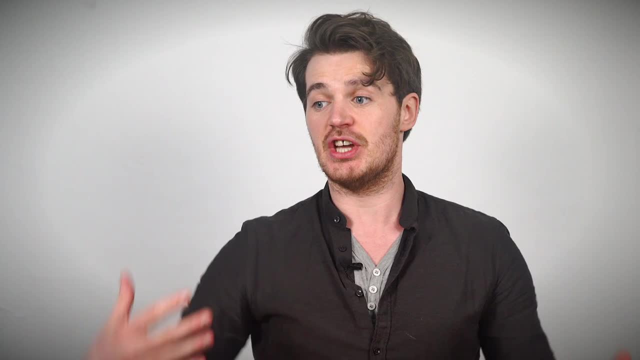 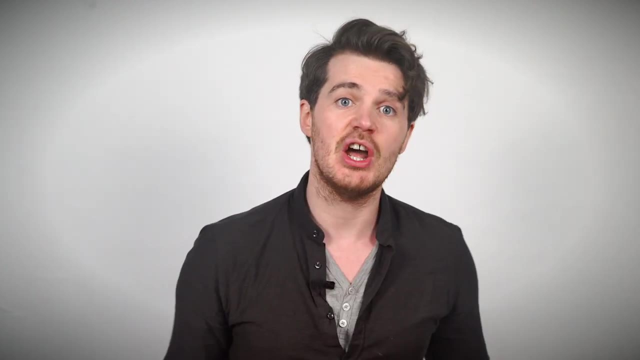 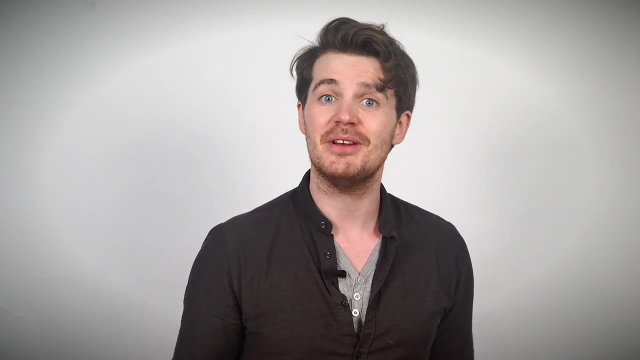 focusing on how much I hate you know that feeling I get during my exercise. I focus on how good I feel after my exercise. In the evening I always do the washing up. Generally, I do this for two reasons. One is that it makes Julia happy because she hates doing the washing. The other one: 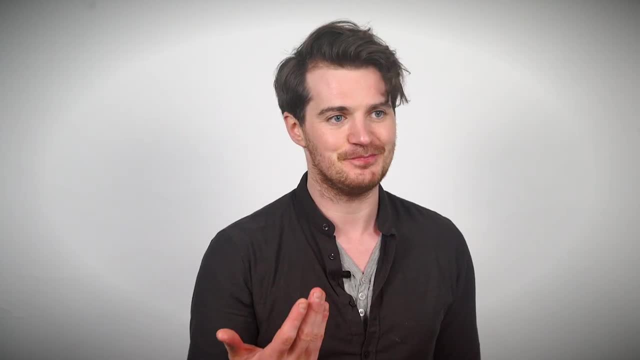 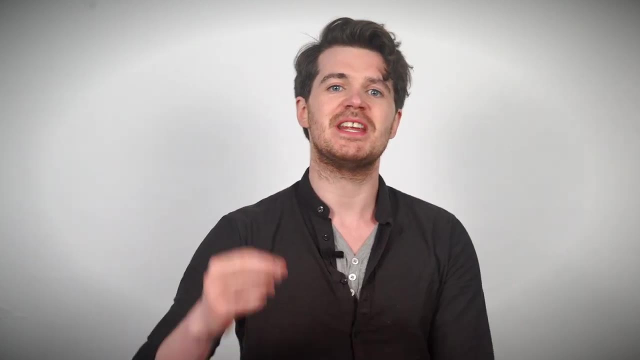 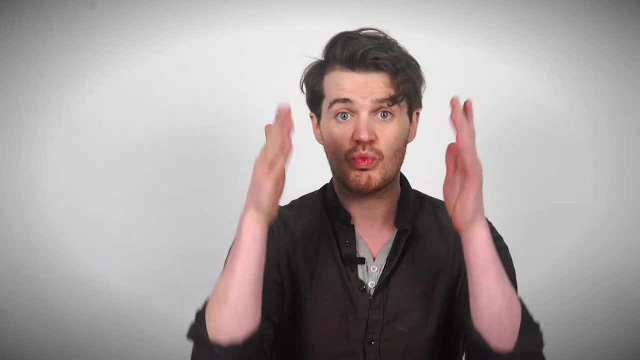 is that making Julia happy makes me happy. But there's also. I get to listen to a chapter in whatever audiobook I am listening to at that moment in time. Positive framing allows me to sail through the good, the bad and the ugly of my daily activities. It allowed me to write this video. 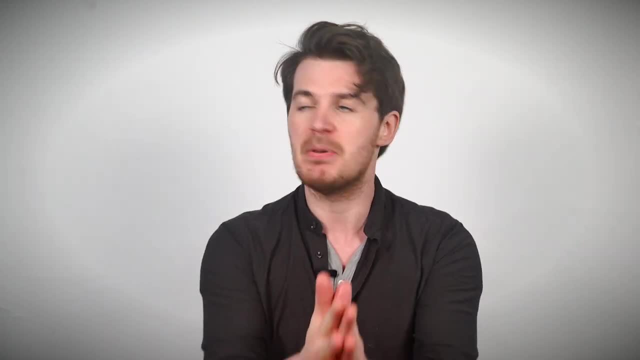 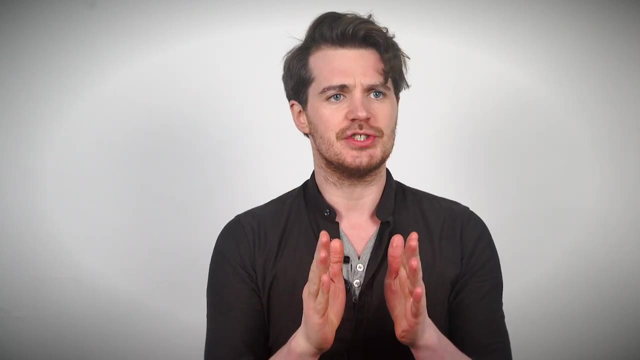 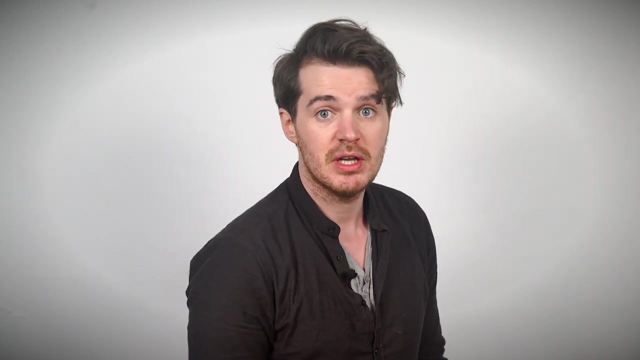 in one sitting, because I knew how good I'd feel once it was completed. Being an optimist is like riding a cloud of possibilities. Or as the playwright Leonard Lewis Levinson wrote: an optimist sees only the dark side of the clouds and mopes. A philosopher sees both sides of the 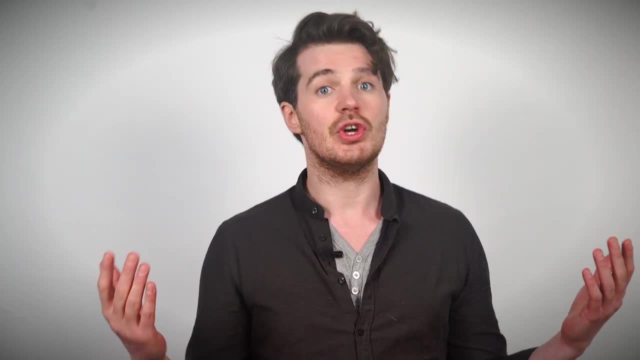 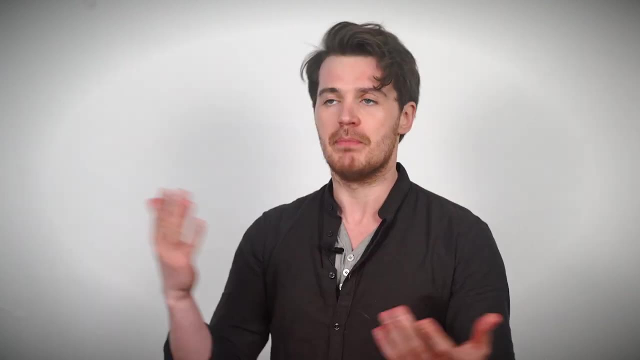 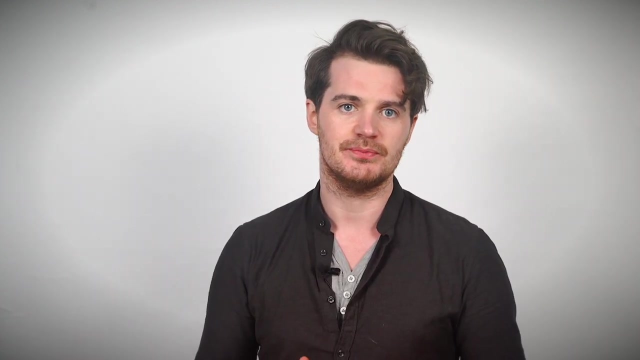 clouds and shrugs The optimist. he doesn't see the clouds at all. He is walking on them. However, sometimes it is good to be aware of the clouds, You know. pack a jacket, take an umbrella. In 1895, Oscar Wilde was sent to prison convicted of indecency. 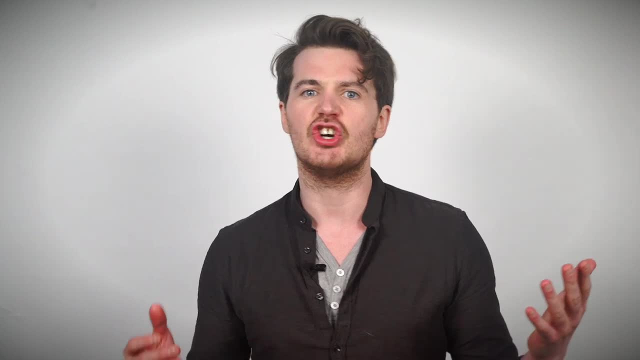 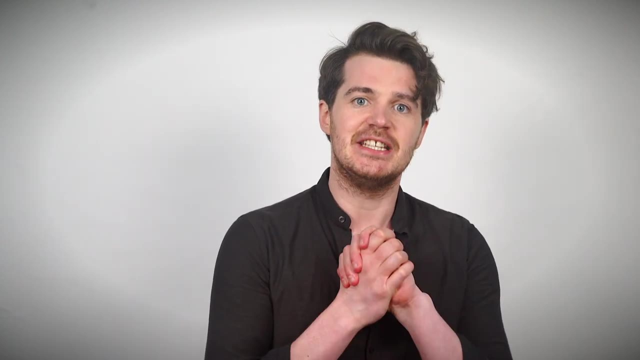 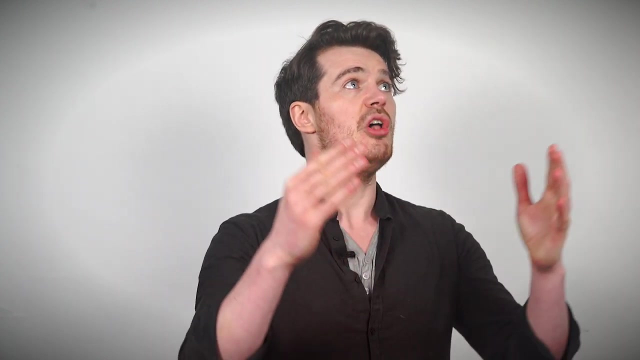 homosexuality. He had lived freely and he got his freedom taken away for it. After his release from prison, living in exile in France in 1900, he died in a hotel room in Paris. His health deteriorated from the years in prison. Either the wallpaper goes in here or I do. where his final words: 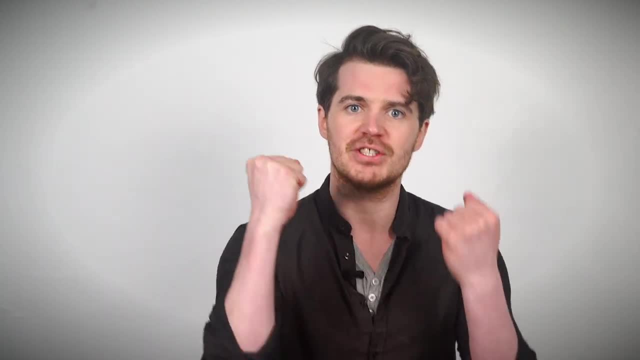 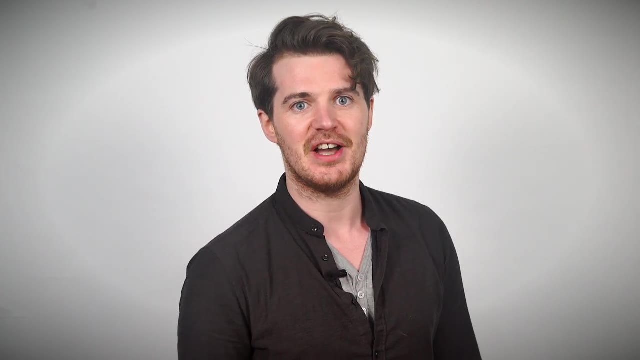 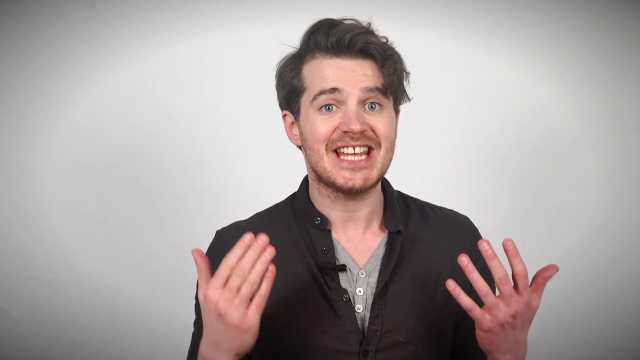 he had an art for framing even the darkest moments in positive light. I'm dying beyond my means, he commented while lying ill in the five-star hotel where he died. But his fall from grace time in prison, loss of his family, his home and even his early death could have been prevented. 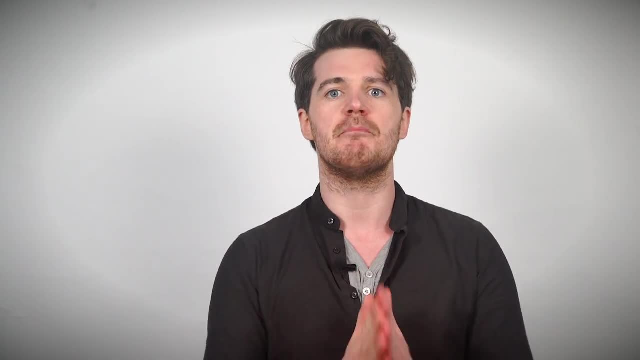 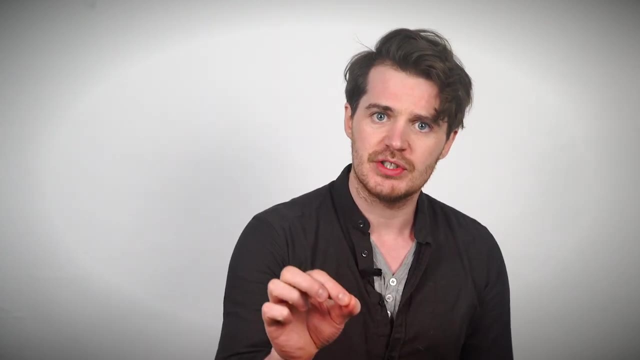 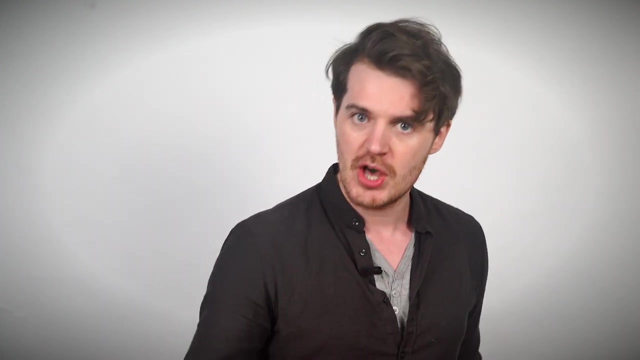 if only he had listened to recognize the warning signs and then build up to his conviction. The lesson here: Our optimistic focus on the flowers shouldn't prevent us from seeing the crap in the park. The crap is there. If you don't see it, you're likely to put your foot right in it. 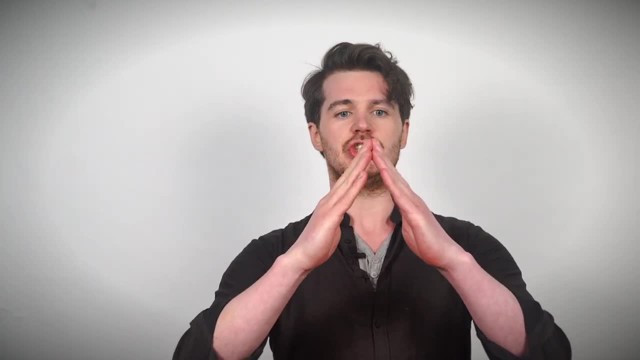 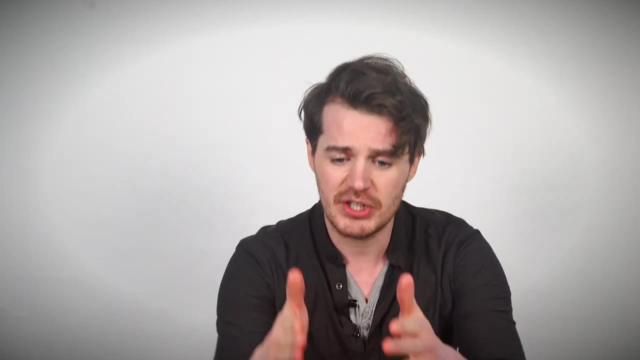 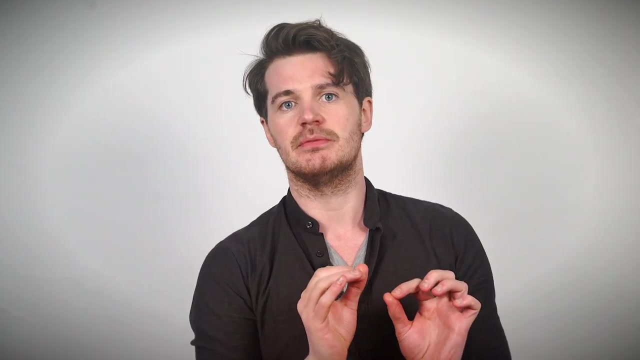 This is the pivot of our little see-saw between optimism and pessimism. The realist, A realist, is a person who accepts the situation as it is and is prepared to take it on accordingly. An American comedian, writer, etc. etc, etc – Bull Myer said that he's a realist. 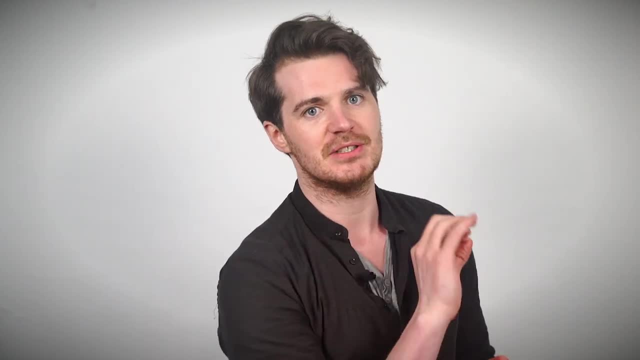 Though he also went on to say that one man's realist is another man's pessimist. But why must one man be anything? Why do men, women need to be defined as anything? why do men need to be defined as anything? One new person has appeared to the picture – an artist – thatarem experiments so many things. one decision that a man receives from history, someone else has got to take a helping hand from it. That other person might have grown men in that personal situation, or maybe not that personal situation: a person might have experienced Lift being in LA. 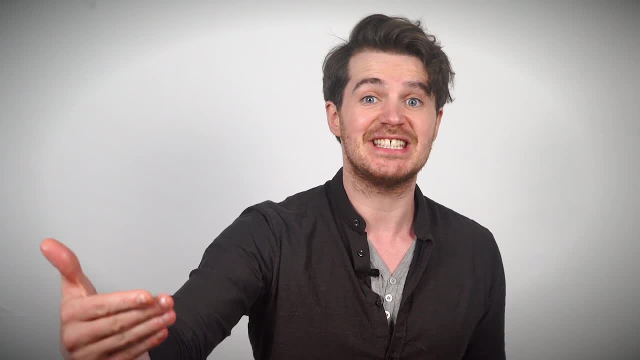 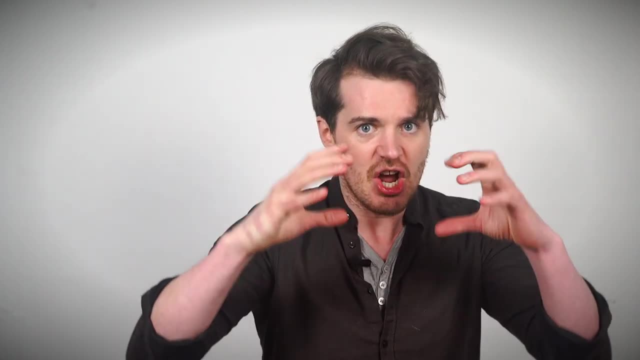 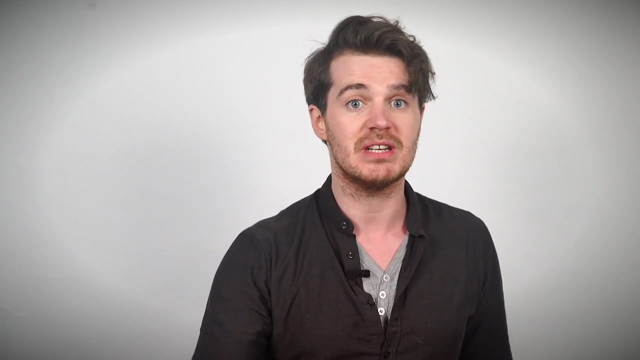 Why do men, women need to be defined as anything? Why do we define ourselves as realists, pessimists, optimists: By defining ourselves, we shrink the frame of our world, we miss out on the details in the park we are walking through and we leave our path open to stepping on some nasty stuff. 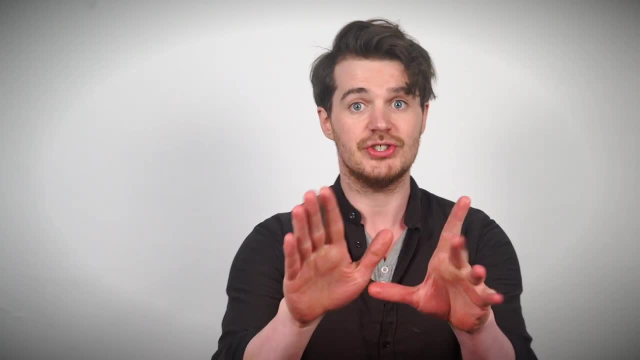 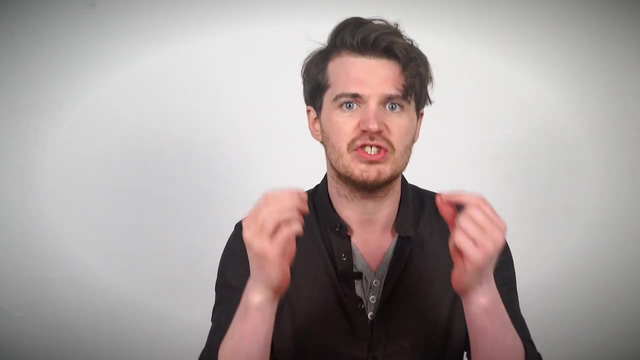 If you decide to indulge in optimistic framing- which you should- you needn't define yourself by this activity. It is a tool and it should be used, like any other tool, for the purpose of improvement, namely the improvement of your life, and it should be used in conjunction with that. 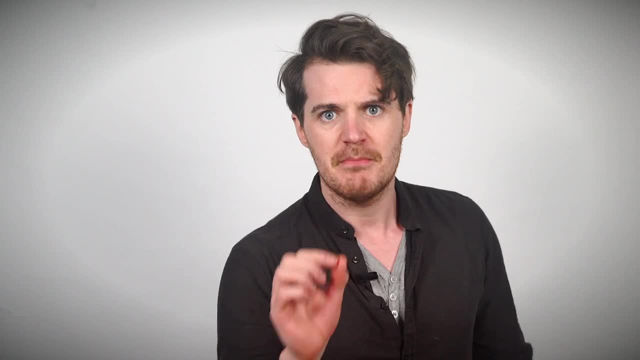 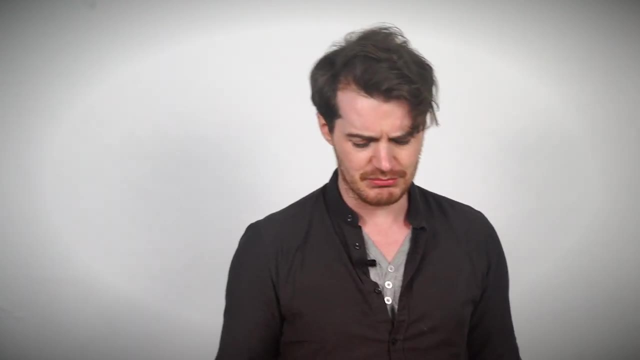 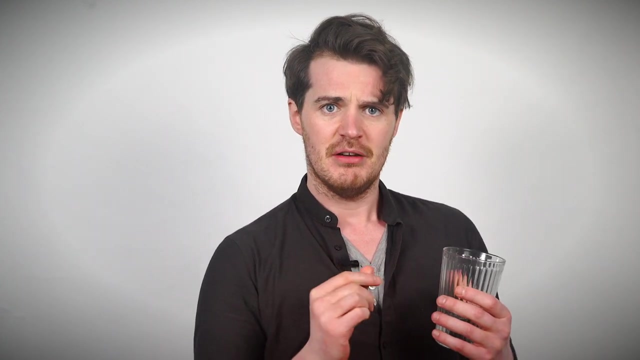 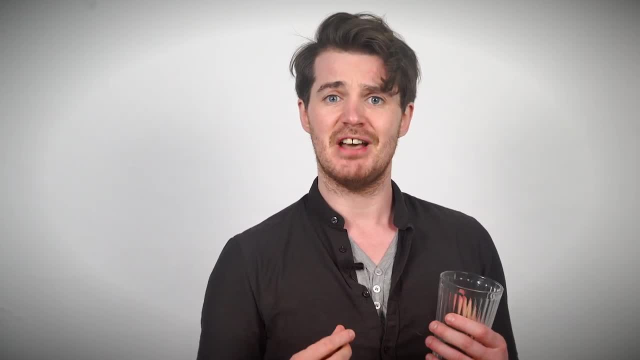 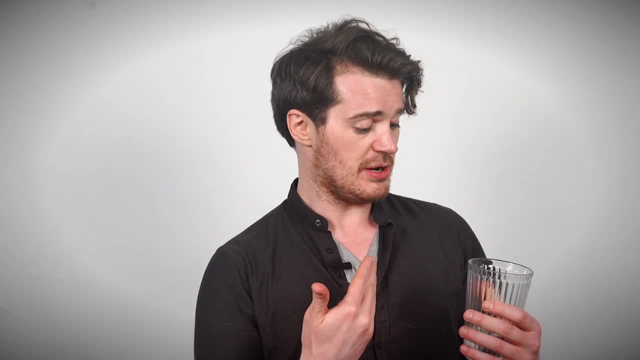 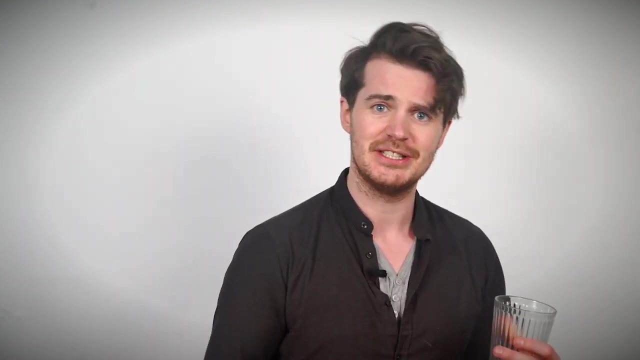 I don't know, Maybe it's better, if it's close to closing time and it's last orders, to consider if it's your round or not. If it is your round, then I would say this is definitely half-full, But if it's their round, then it's positively drained.